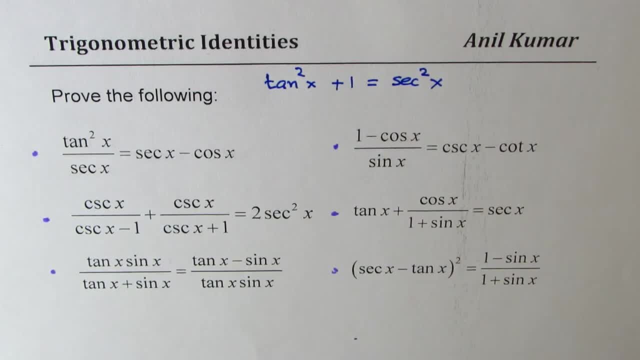 minus 1 will solve your question In first two. you'll find those to be very straightforward. However, the next four involves a lot of manipulation and tricks. So some more ideas let me give you before you begin Here. we have secant x minus 1.. So the common denominator we use 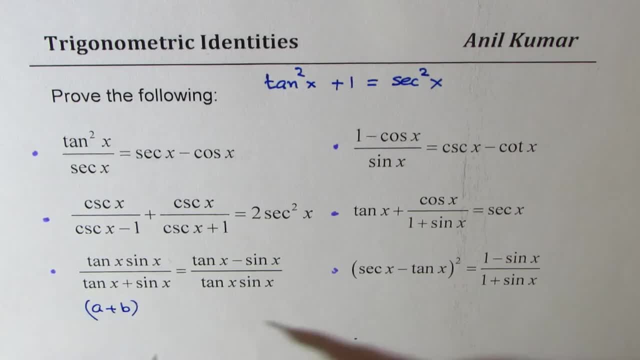 the formula a plus b times a minus b: A plus b equals to a squared minus b squared correct. So that will be applied and I hope you remember what is a minus b whole squared equals to. That is equal to a squared minus. 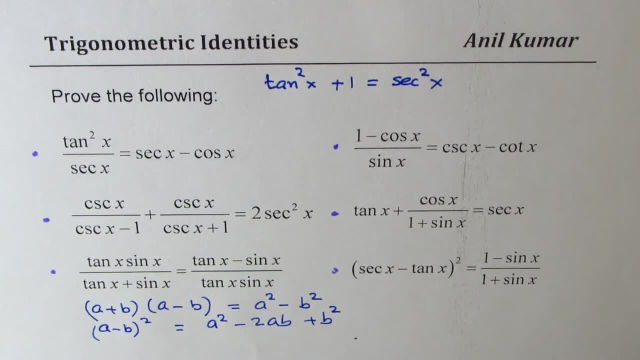 2ab plus b squared. Now I think you are armed with everything you need. You can actually start solving them, rather proving these identities, and then look into my suggestions. So let's start taking the very first question Now. these two are very simple examples, straightforward. 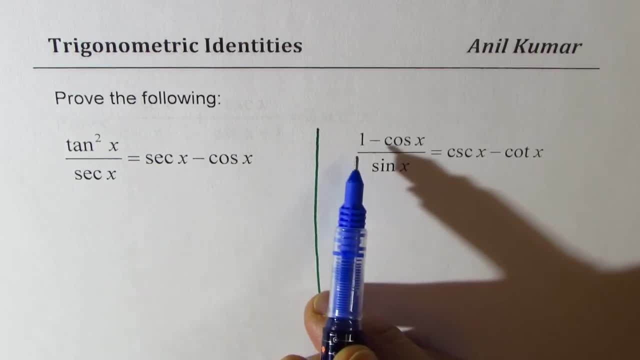 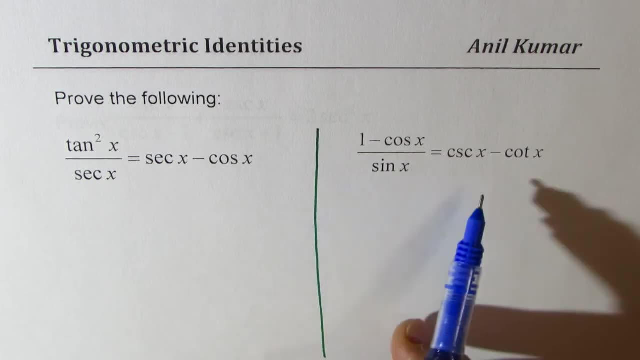 application. So let me begin with the second one: 1 minus cosecant x over sine x. In proving identities, you should start from one side and prove the other one. At times, if they are complicated, you would start from both and prove that both are equal to the third. 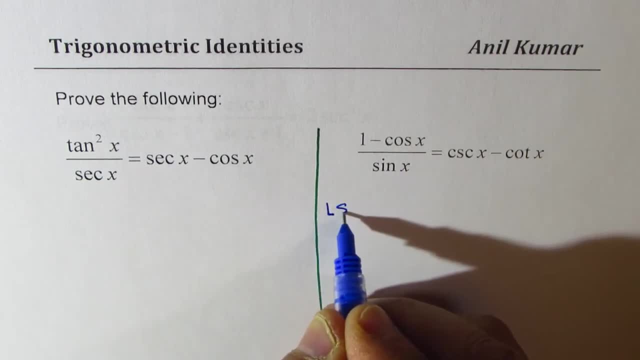 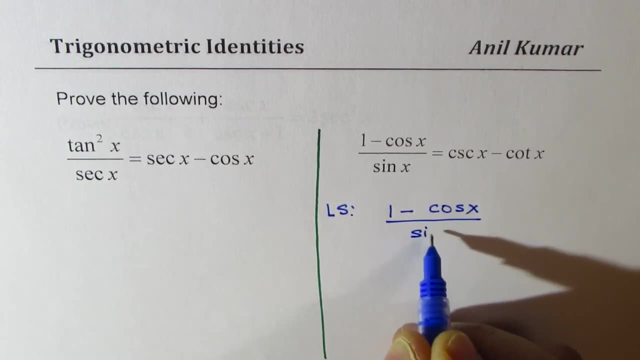 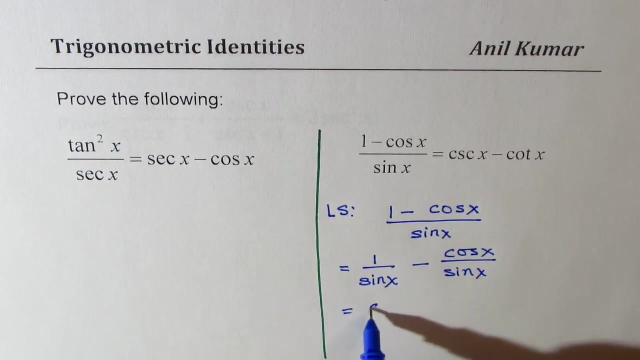 thing right. So in this case we'll start from the left side. So the first one is given to us as 1 minus cos of x, divided by sine of x. If I just rewrite 1 over sine x minus cos x over sine x, what do I get? 1 over sine x is cosecant x and 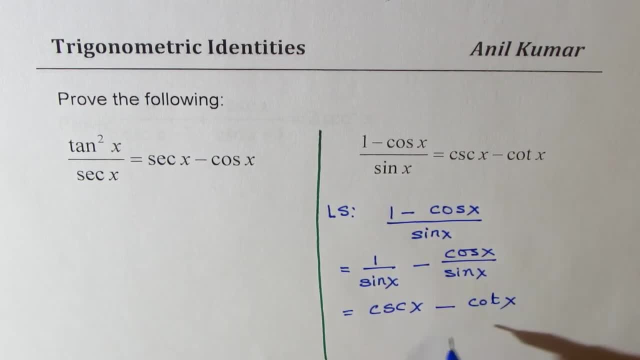 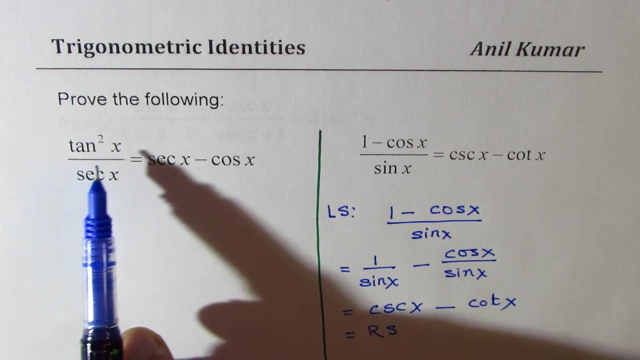 cos over sine is cotangent, So we get the right-hand side. Do you see that? As simple as that. So this is straightforward, and that is how some identities can be proven. Now here second identity: tan square x over secant square x. Whenever you see tan square. 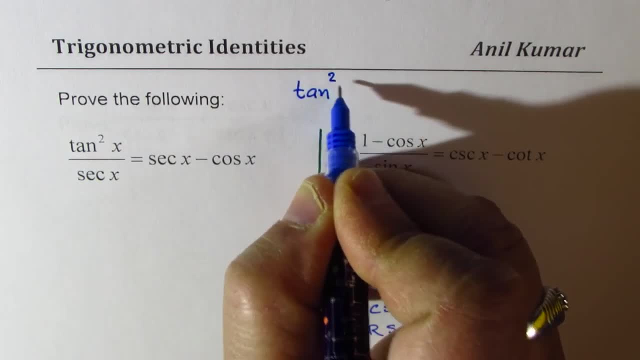 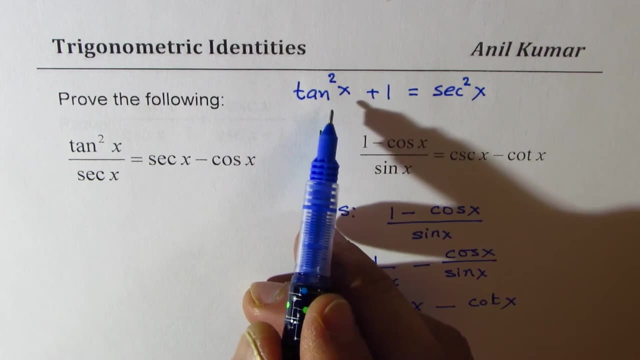 x. you should be reminded of this Pythagorean identity, which is: tan square x plus 1 is equal to secant square x. correct? Now, from here you could write: tan square x is secant square x minus 1.. Right. 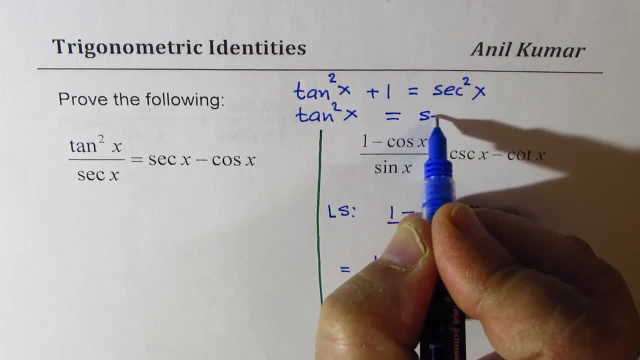 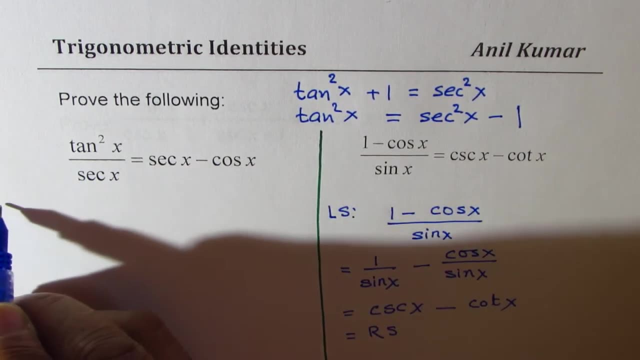 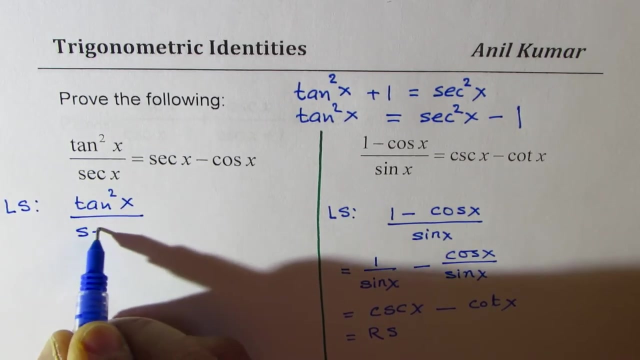 Let's rearrange this. Rearrange right, So it could be written as secant square x minus 1.. So now we can easily solve this. Now, here also, let's begin with the left side, which is tan square x over secant x. Now, since we saw that tan square x can be written as: 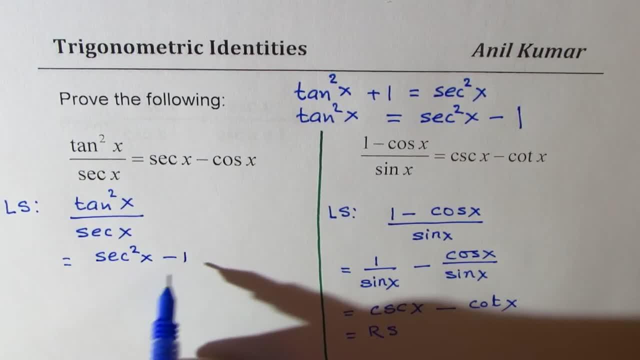 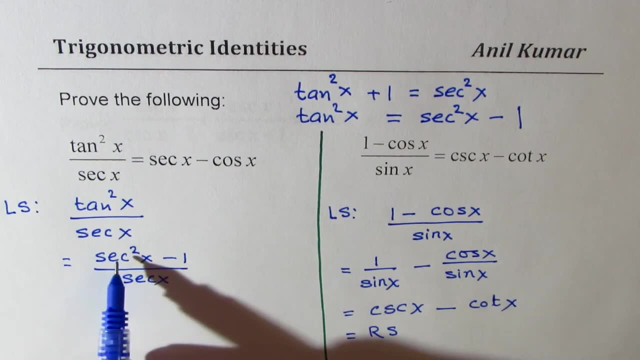 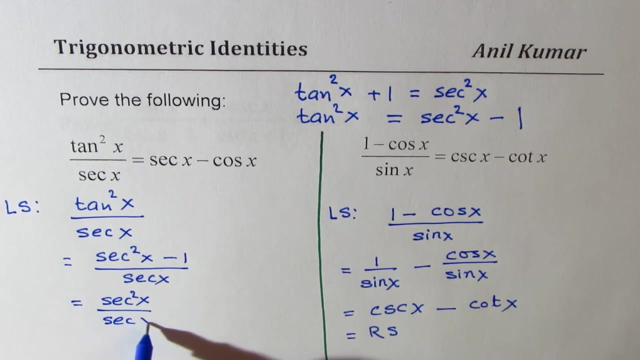 secant square x minus 1, so let's replace it with that and see what do we get. So we get. so what we get here is secant square x over secant x. Let me rewrite this: We get secant square x over secant x minus 1 over secant x. Now, secant square x over secant. 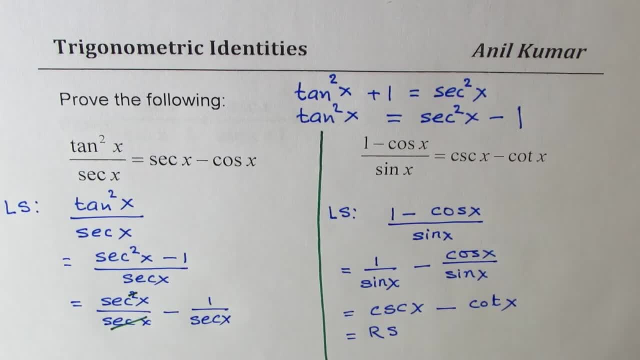 x could be simplified. One of them goes: and what are you left with? You get secant x on the left side. I mean the first term and the second is 1 over secant, One over secant, which is cos. So we get minus cos x. Correct, So we have shown that left side is equal. 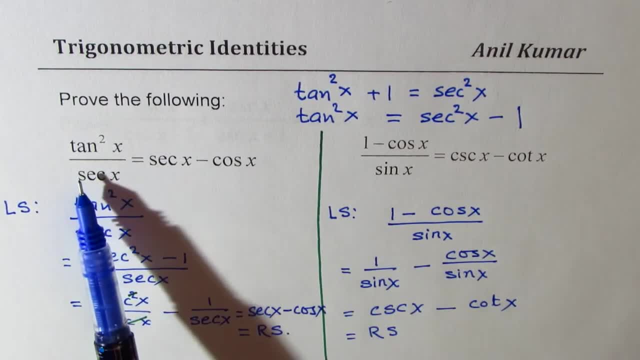 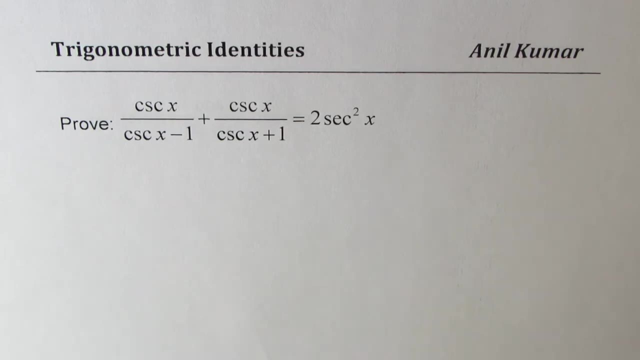 to right side. So the whole idea here is to prove that both the sides are same, and then we say that we have proven the identity Right. So that's the concept, And now let's begin with the intricate questions which involve some more steps to solve. So here, 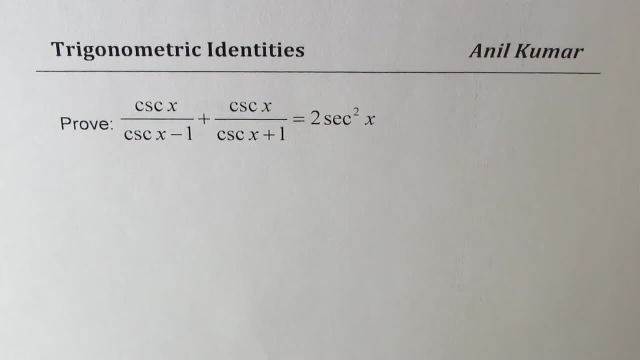 is another question for you. Cosecant x divided by cosecant x minus 1 plus cosecant x divided by cosecant x plus 1 equals to 2 times secant square x. I'd like you to pause the video, prove this identity and then look into my suggestions. Now, in this identity, we should: 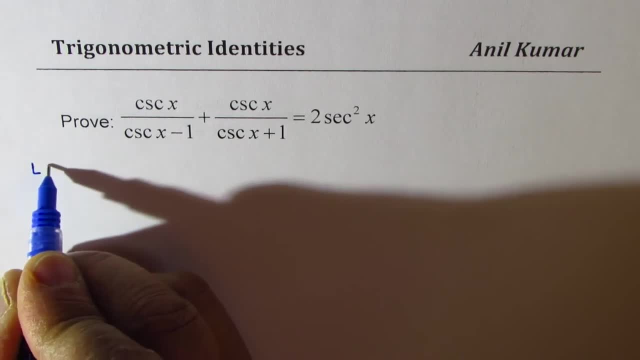 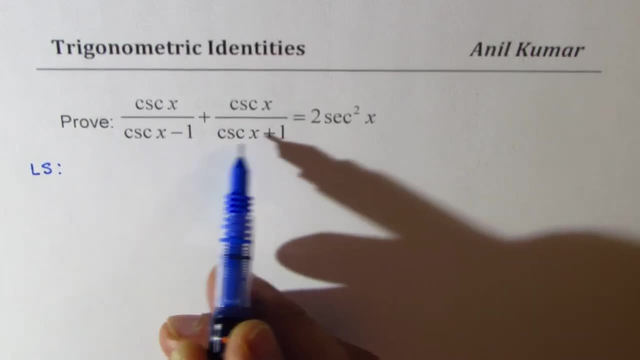 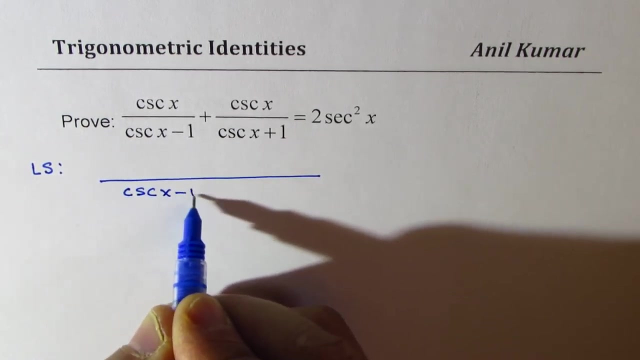 begin with left side. It is complicated, So therefore it is simpler to simplify. Correct. So let's begin from the left side and we'll take the common denominator. So the common denominator will be product of Cosecant x minus 1 times cosecant x plus 1.. Correct, So that product becomes the common. 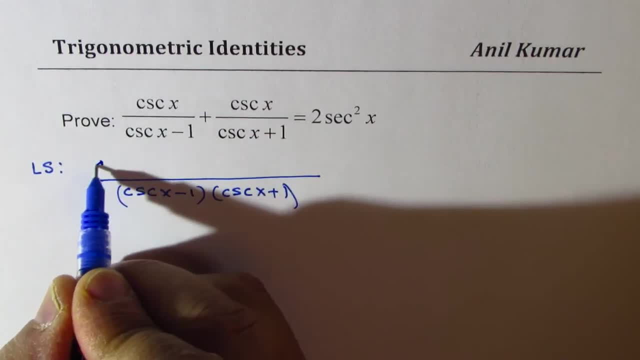 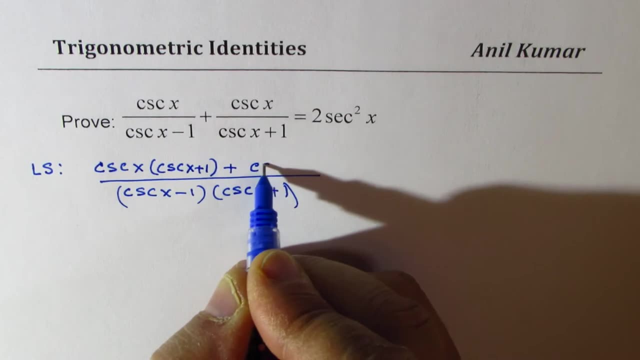 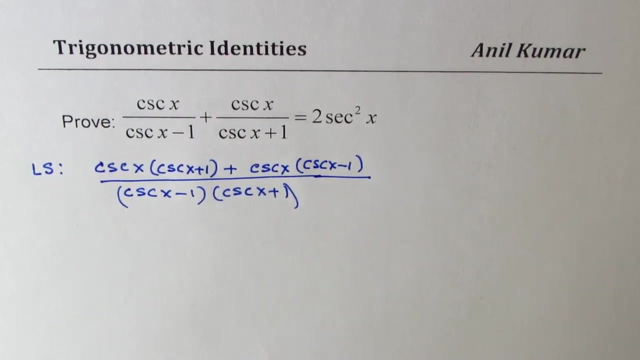 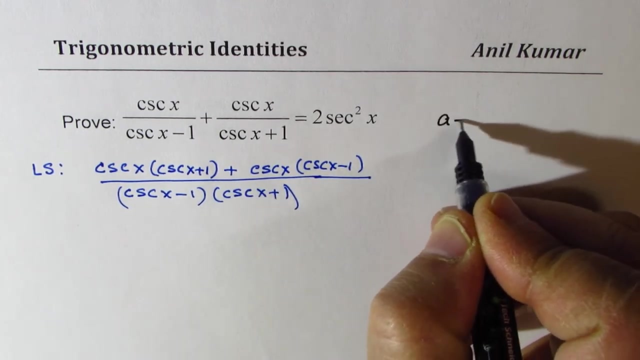 denominator. Now we'll cross multiply, So we'll have cosecant x times cosecant x plus 1 plus cosecant x times cosecant x minus 1.. Now the denominator here is kind of the form of a plus b times a minus p, Right, So we have a plus b times a minus b When you multiply. 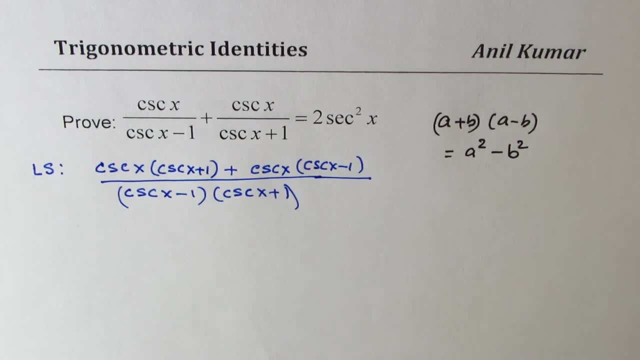 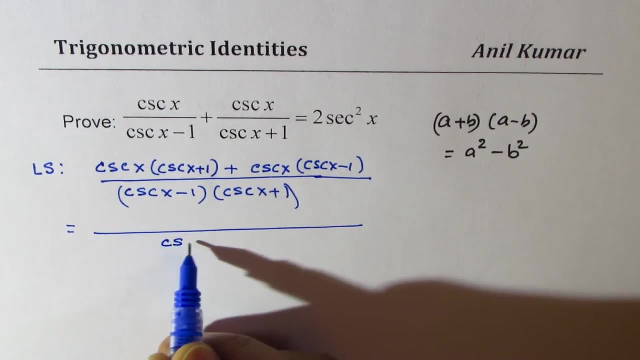 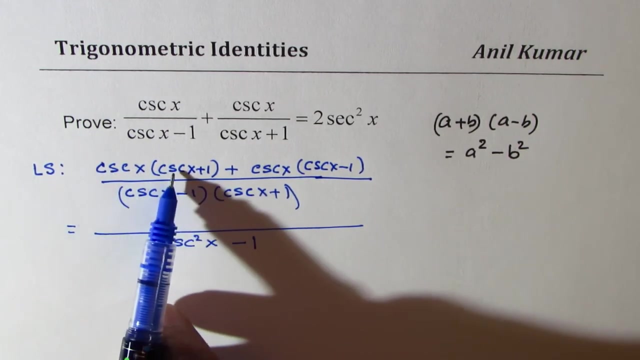 you get a squared minus b squared, Perfect. And therefore I could write this left side now as denominator being cosecant squared x minus 1.. And in the numerator we have cosecant x times, so we'll apply the distributed property and expand, So we get cosecant squared. 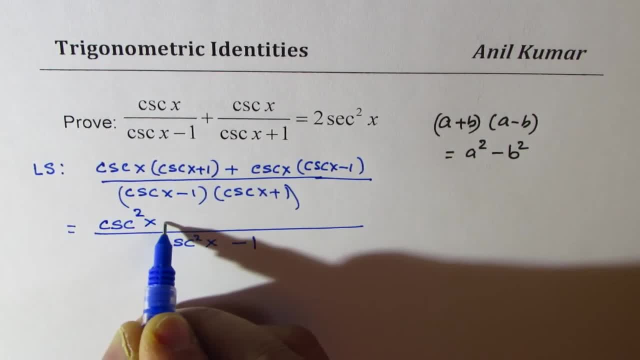 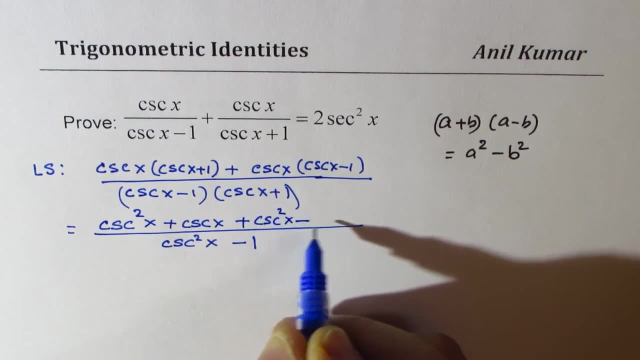 x times cosecant x minus 1, x is equal to 1.. And we'll multiply that by cosecant So we get cosecant x times. So we'll apply the distributed property and expand, So we x plus cosecant x plus cosecant square, x minus cosecant x. correct, That's what we get Now. 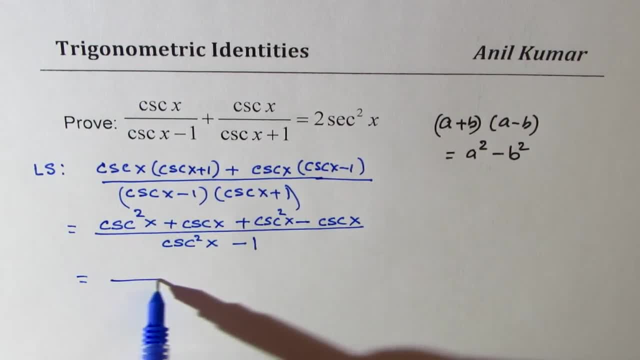 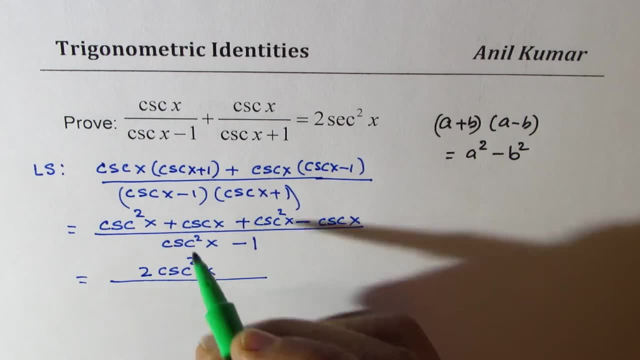 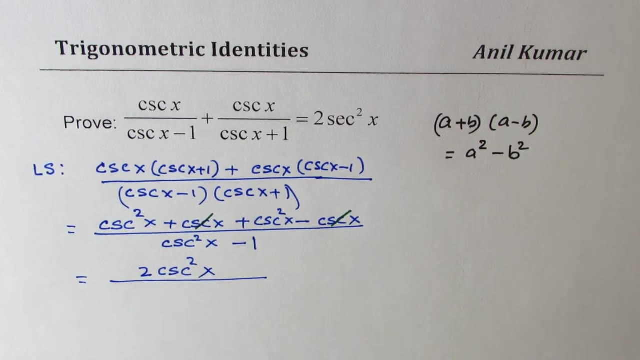 you can clearly see that these two terms cancel away. So in the numerator we have two times cosecant square x, right? So let me cancel these two positive and negative terms. Now how can you write the denominator? So I hope you remember another trigonometric identity. 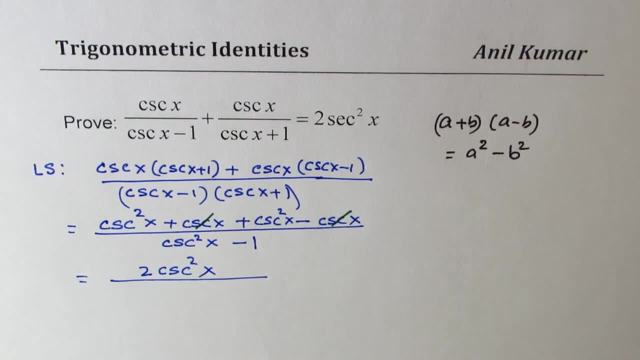 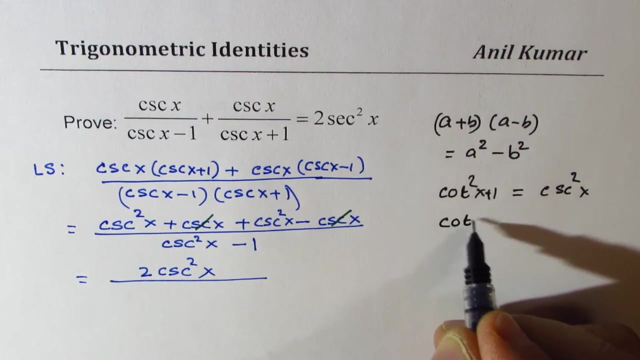 which relates cotangent with cosecant right. So we have cot square x plus 1 equals to cosecant square x. Now if I take 1, I mean plus 1, so if I take 1 on this side, what do I get? I get cot. 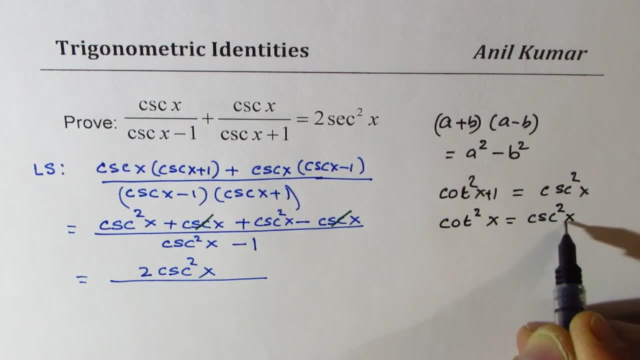 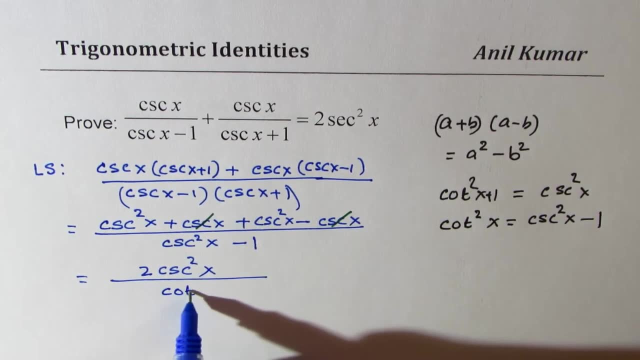 square x equals to cosecant square x minus 1.. So cosecant square x minus 1 in the denominator could be written as cot square x. Perfect. Now we need answer as 2 times secant square x. We already have a 2 here, So let's write. 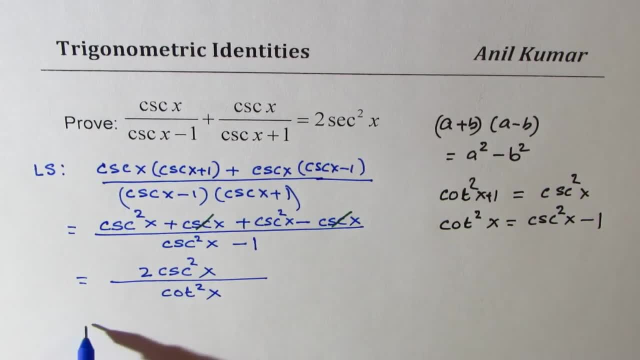 them in cos and sin. So we could rewrite this as 2 times. Now what is cosecant square x? It could be written as 1 over sin square x, correct? Now How to write cot square x? Cot is cos over sine. 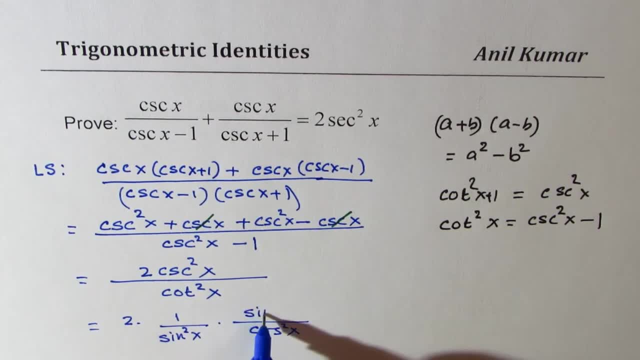 So cos square x in the denominator and sine square x in the numerator. So we have written cot square x. I hope you appreciate this technique. We are avoiding layers of fractions. At times you will see four layers of fractions to rewrite this. But no, we should write like this: 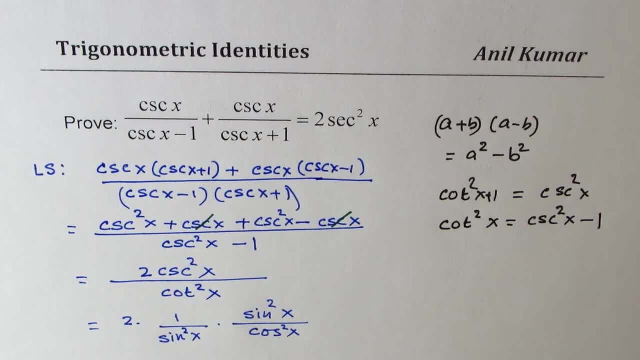 This is much simpler and better to understand Now from here. clearly, these two terms cancel away, and what are we left with? We are left with what we need, which is two times one over cos square x, and you know, one over cos x is secant. 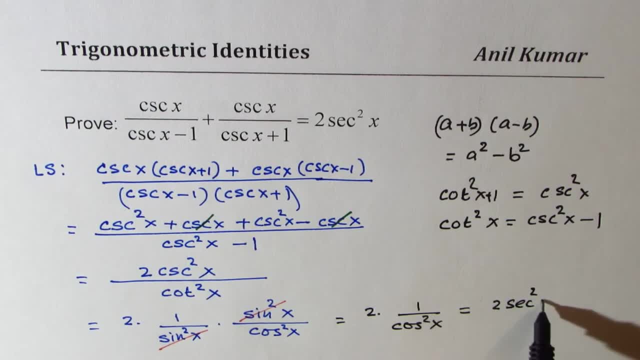 So one over cos square x will be secant square x, and that is what we wanted. So that is how you prove this identity. So you can see that many steps are involved in proving this particular identity and that is why It is slightly more difficult than the previous problems. 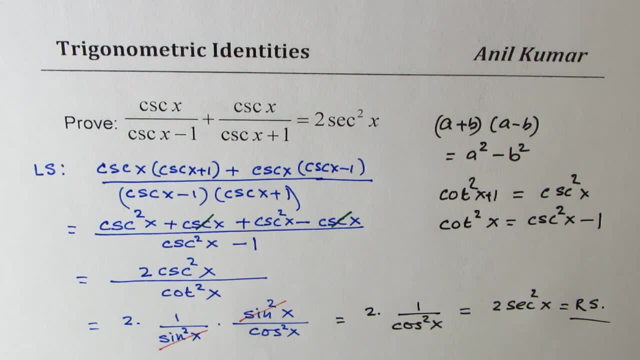 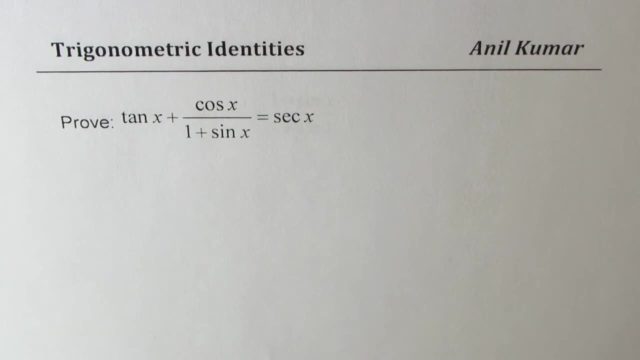 So as we move on, we are taking more challenging questions and I hope you find interest in solving them and learn from them. So now let's pick up the next trigonometric identity. Now we need to prove tan x plus cos x divided by one plus sine x equals to secant x. 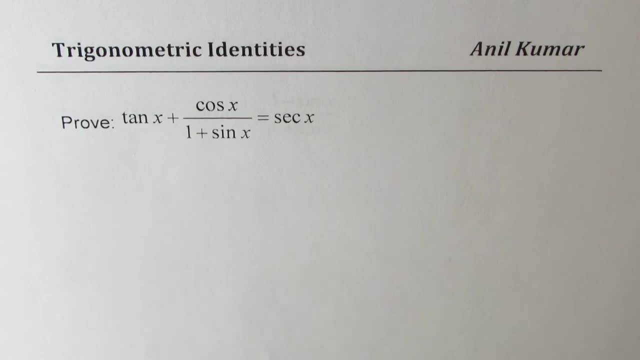 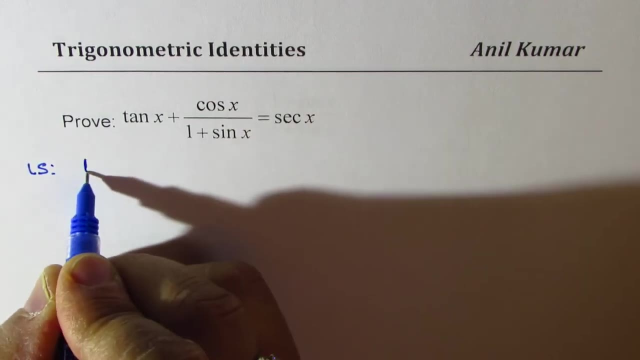 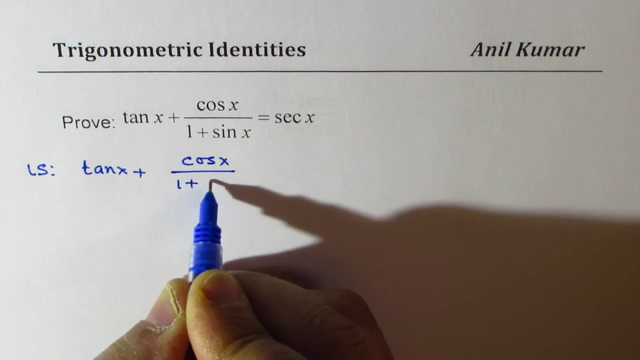 Now this is actually a challenge question. How do we solve this? Well, There is a strategy involved here. We will actually begin with the left side and we will rewrite this as tan x plus. we have this function: cos x over one plus sine x. 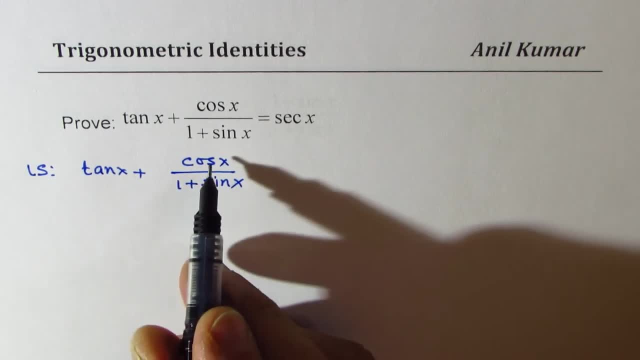 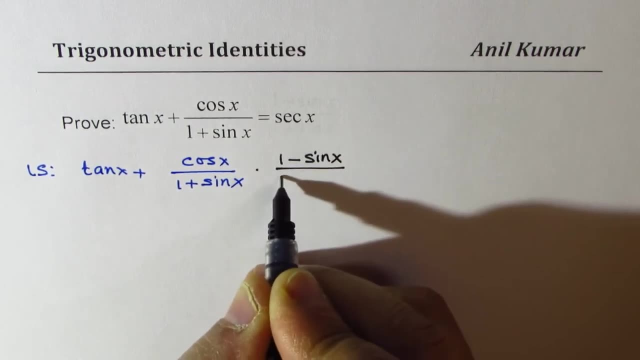 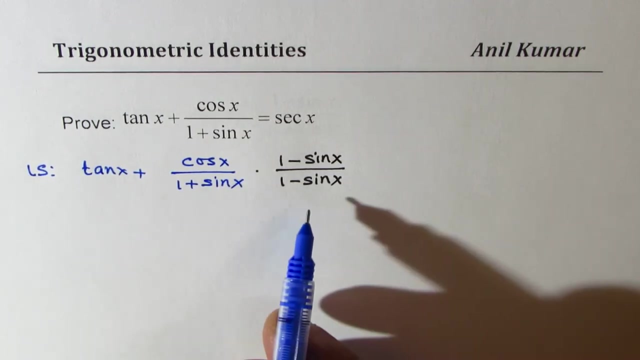 Now, the trick involved here is that we could rationalize one plus sine x by multiplying this by one minus sine x and also dividing by one minus sine x. You see, this step Now, This is an extremely critical step That really helps you to solve this particular identity. 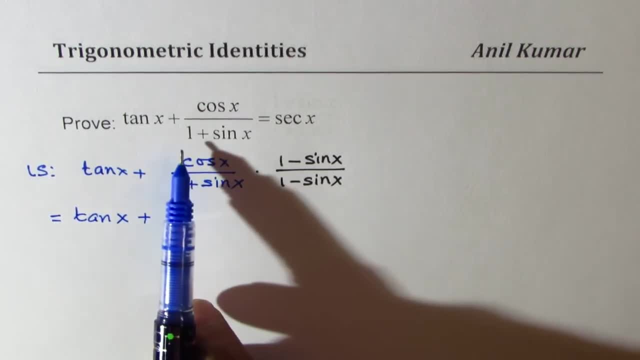 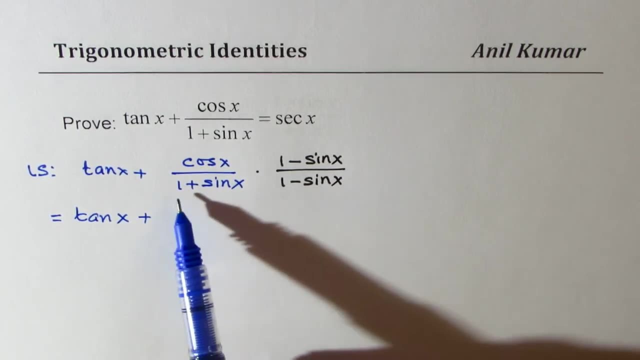 So I would like you to remember that many times when you see a function like one plus sine x or one plus cos x, you could multiply by that. So if it is one plus cos, it will be one plus cos over one plus sine x. We call it rationalization. 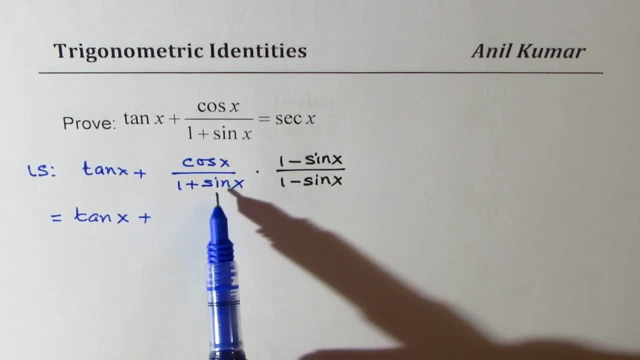 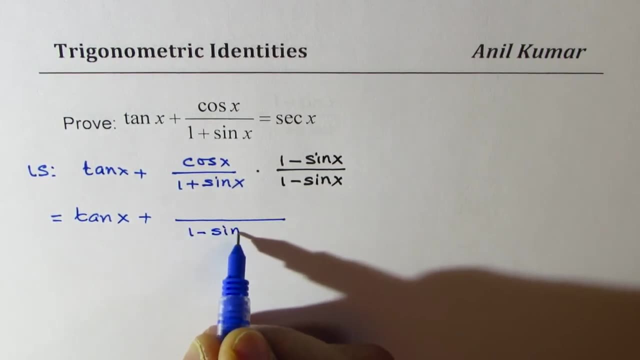 Now then we know what the denominator is: One plus sine x times one minus sine x. One minus sine x is one minus sine square x, One minus sine square x, Correct, So we again applied that sum into difference formula: Difference of squares. 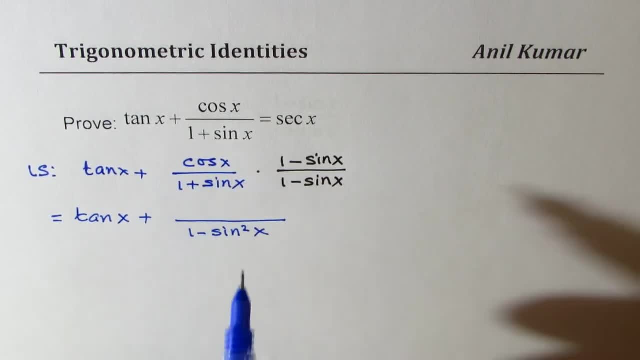 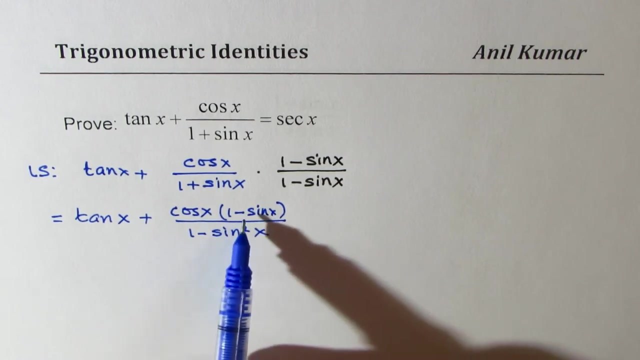 Right, One square minus sine square x. And here we have cos x. Don't expand the numerator One minus sine x. That's kind of interesting and always to be taken into account. Now, the idea is That in the denominator We'll get: 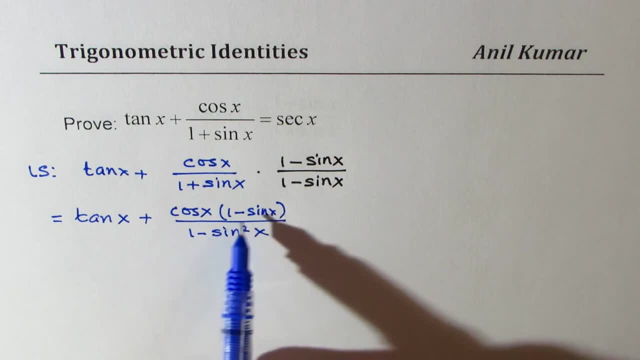 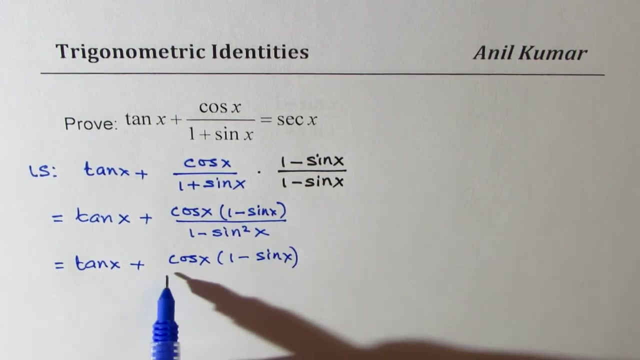 One minus sine x as a factor. Cancel them out And simplify. That's the idea. Okay, So we have tan x here. So let me write down tan x plus cos x. Keep the numerator as such. If you expand that, then you are moving away from the solution. 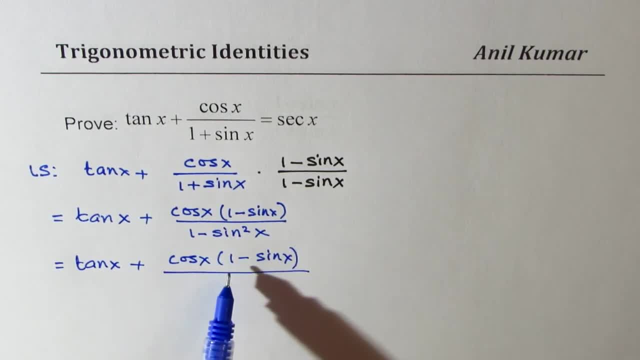 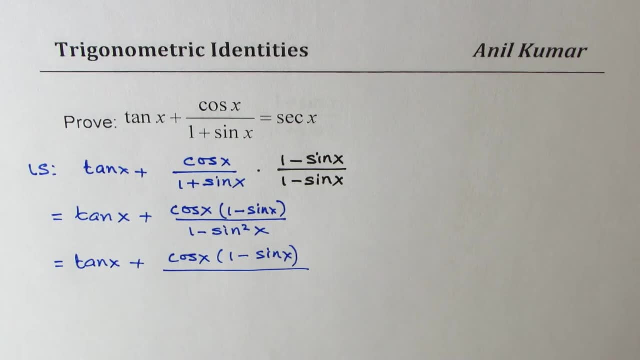 And what is one minus sine square x? Well, we do see a factor here which is one minus sine x. We see cos x here, But secant means we need cos in the denominator Perfect. Therefore, one minus sine square x could be written as cos square x. 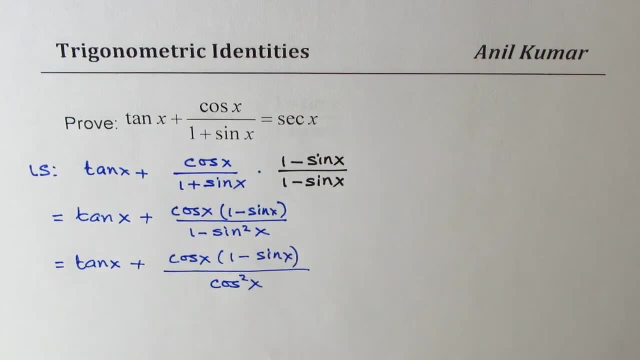 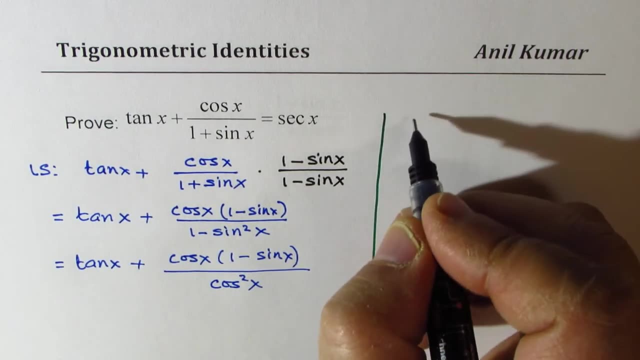 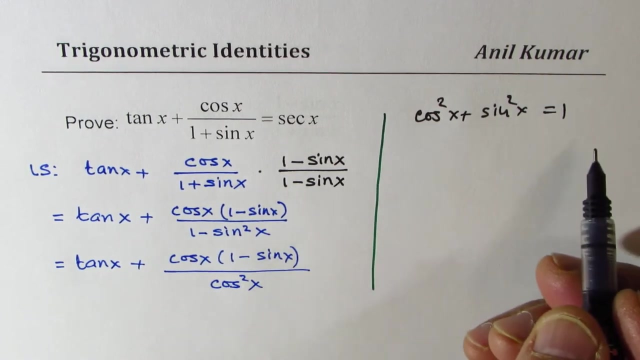 So that approaches to our solution: secant x. Now, how did I get that? Okay, Let me just show it here. You remember the Pythagorean identity, which is: cos square x plus sine square x equals to one. So in trigonometric, this is your basic identity. 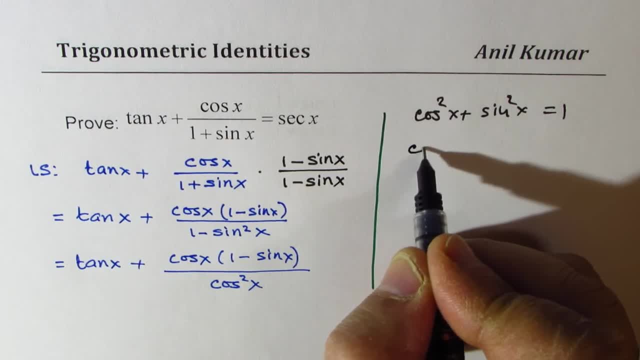 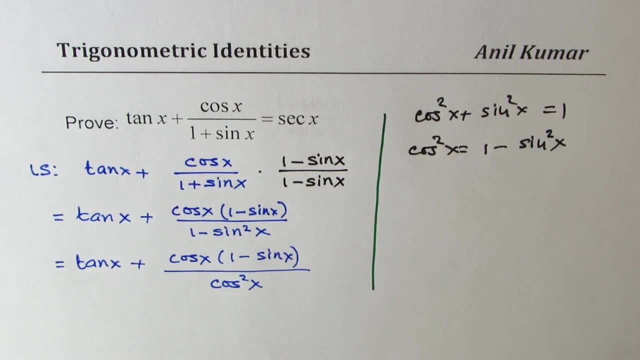 So if I take sine square x to the right side, I get cos square x equals to one minus sine square x. Simple as that. So that is how you get it Perfect. Now you can simplify by cancelling one of these cos, Correct? 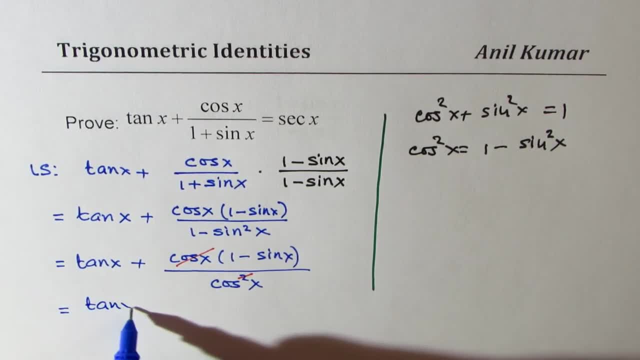 So what is remaining there? It is tan x plus one over cos x, minus sine square x. Perfect, So you get tan x minus sine x over cos x. Do you see that part? So one over cos x is secant x, which you wanted and you don't want this tan. 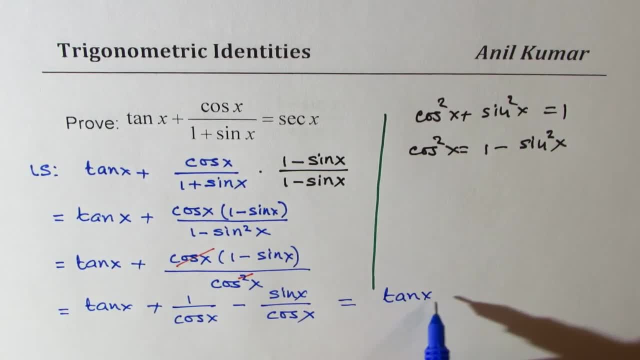 And fortunately what you have here is tan x plus one over cos x can be written as secant x, and sine x over cos x is tan x. So you get tan x minus tan x. They cancel away and you are left with secant x. 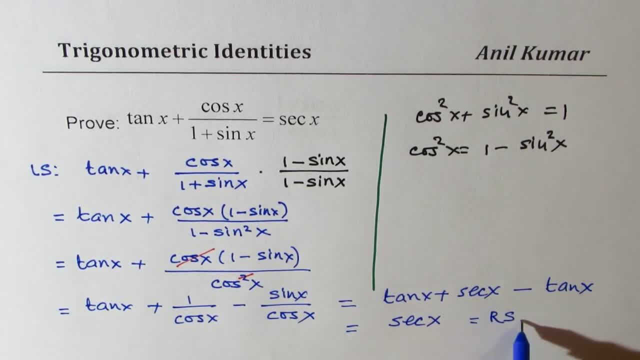 Do you see that part? Perfect. The right side equal to the left, which is the right side? Perfect. So that is how you prove. So you are shown that left side is equal to right side. so this is the strategy with which we are going to work. 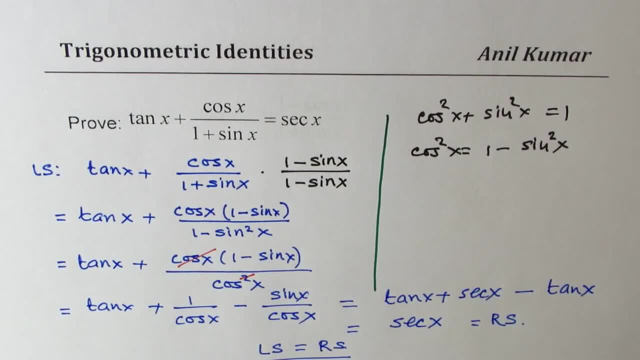 Now critical step here is not to disturb tan x, as we see that later one it gets cancelled by itself. Do you see that part? And that makes this question extremely interesting. Perfect, So I hope you're learning as you move on with this interesting questions. 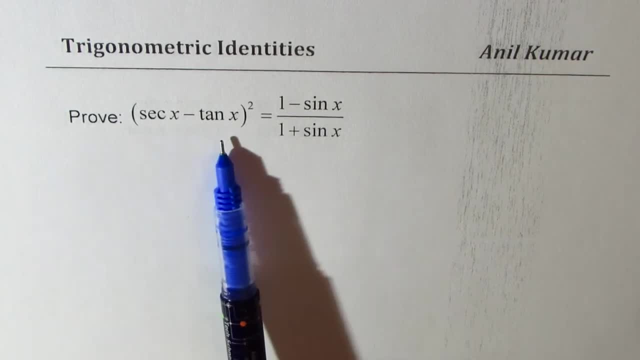 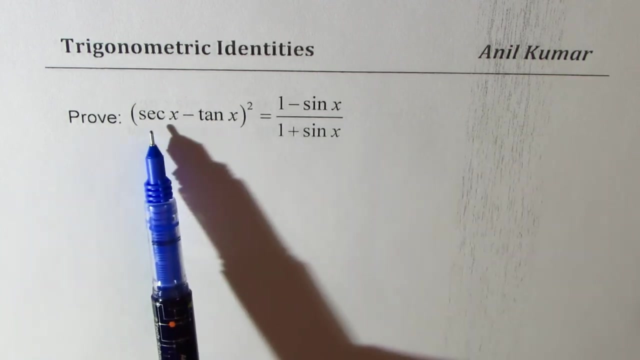 Perfect. Now here is another one. We have secant minus tan x. whole square equals to 1 minus sine x over 1 plus sine x. Now in such questions you could do a couple of things, That is, you could rationalize this side and begin with, or you could work with this. 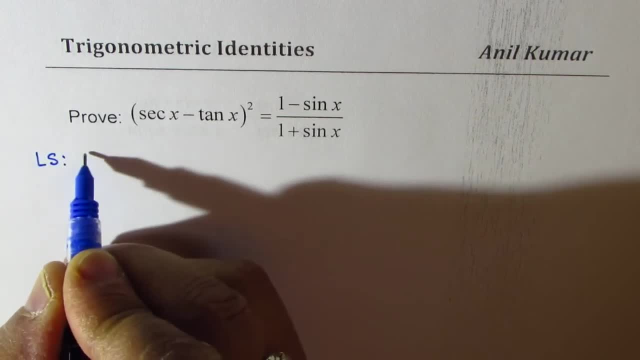 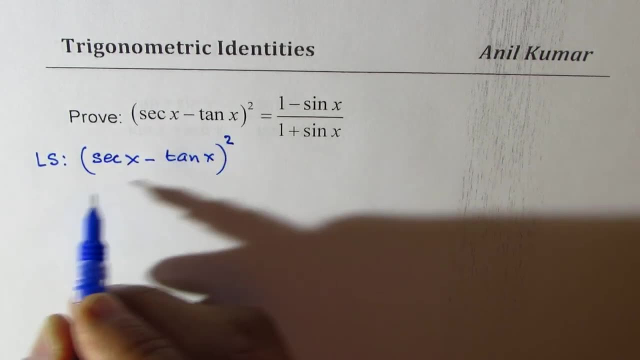 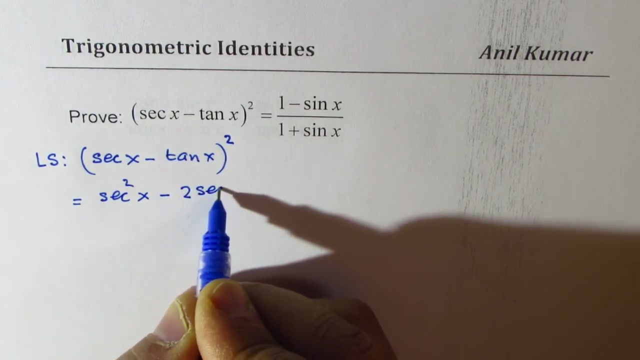 So let's prefer to do the left side. So we have secant x minus tan x whole square. And if I expand this, what do I get? I get secant square x minus 2, secant x, tan x plus tan square x. 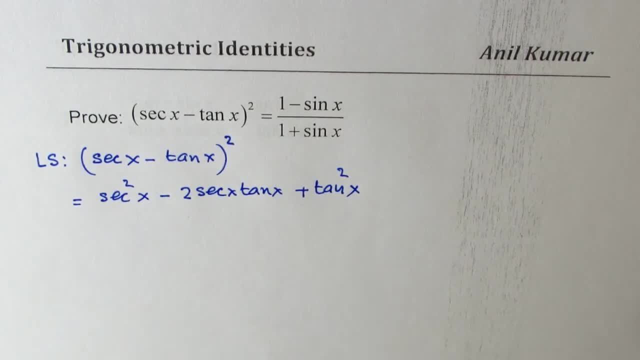 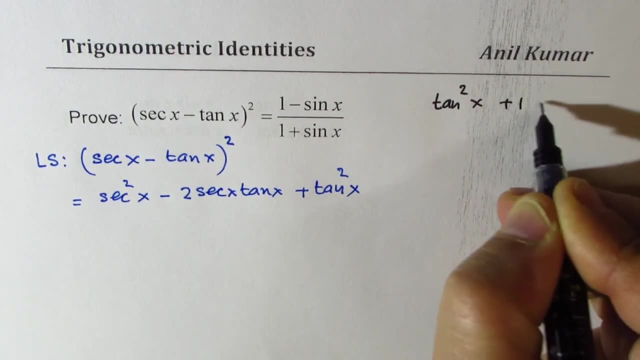 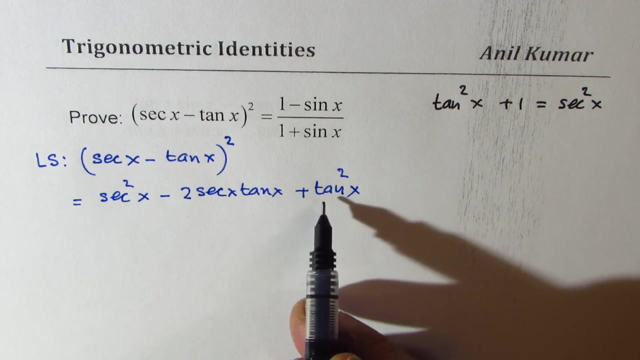 Correct, That's what we get, And we know one formula which relates secant and tan, and that is: tan square x plus 1 is equal to secant square x. So what is secant square x plus tan square x? You, You really don't have any formula relating them. 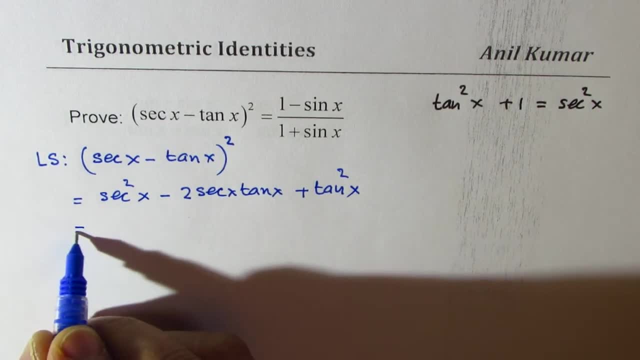 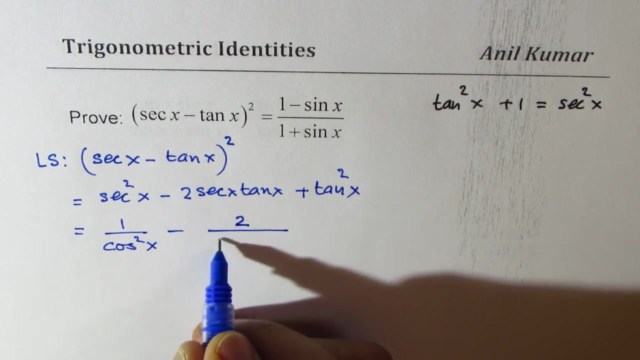 So that really doesn't help you much. OK, So we'll write them in terms of sine and cosine. So we get secant as 1 over cos square x, And here we have two times: secant is what, Secant is cos x and tan x is what. 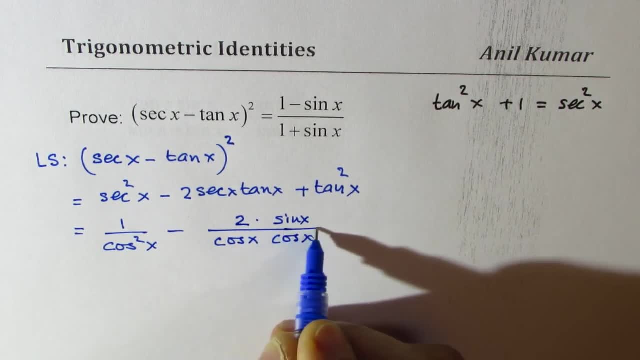 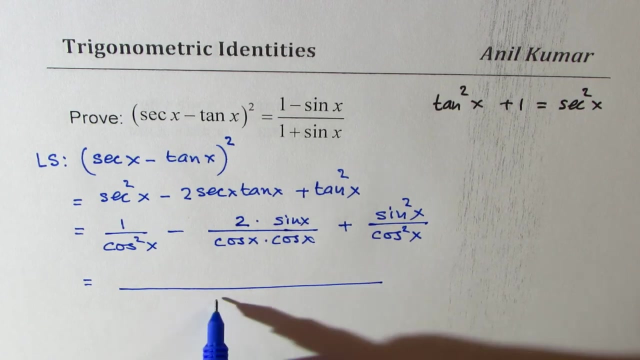 Sine x over cos x, OK, So we again get cos square x. And as far as tan is concerned, we know it is sine over cos. Since it is tan square x, we again get cos square x in the denominator. So we have a common denominator which is cos square x. 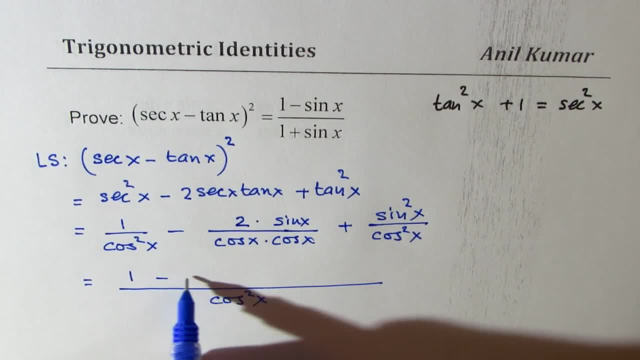 And in the numerator we find we have 1 minus 2 sine x plus sine square x. Now can we simplify this one? I think we can. OK, This is like a perfect square: 1 minus sine x, whole square right. 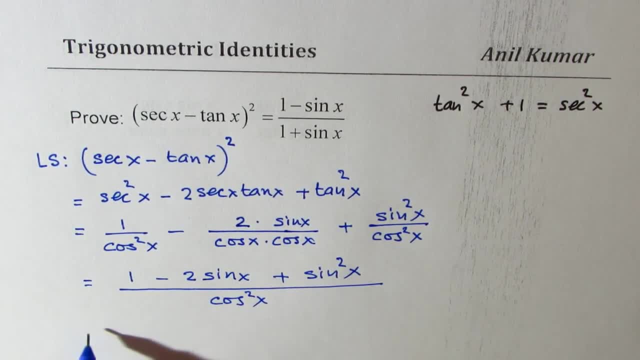 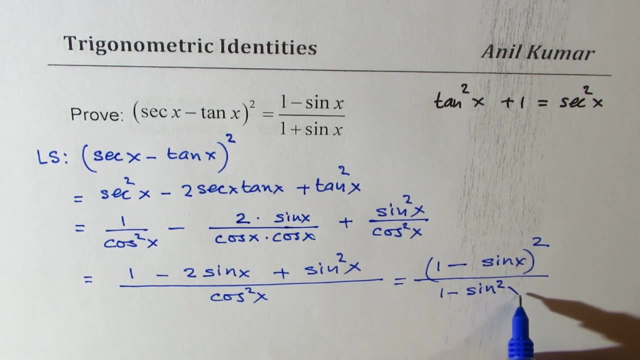 So I could write this as equal to. let me write down here: 1 minus sine x, whole square. Do you see that part? And the denominator, which is cos square x, could be written as 1 minus sine square x, right. 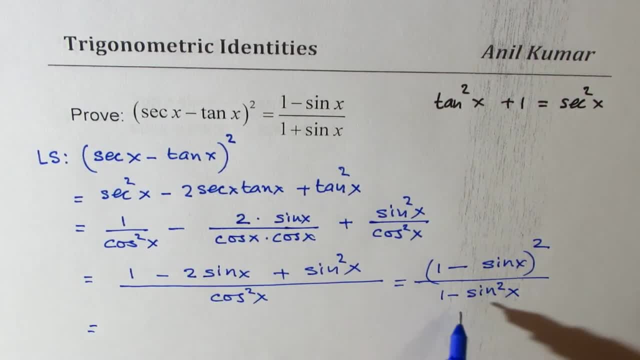 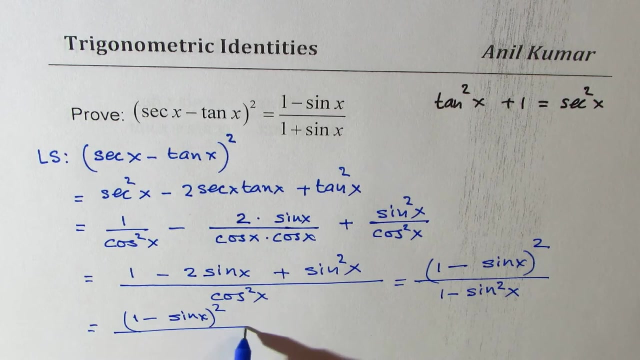 Just as we did in the last video, Now we are going to use difference of squares, right, Right, Just as sum and product of 1 plus sine x and 1 minus sine x. So what we have here is 1 minus sine x whole square divided by 1 plus sine x times 1 minus. 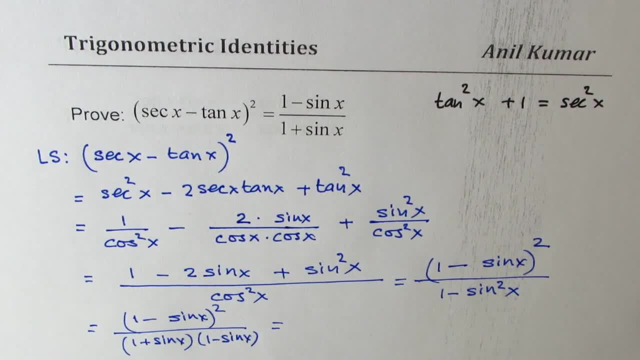 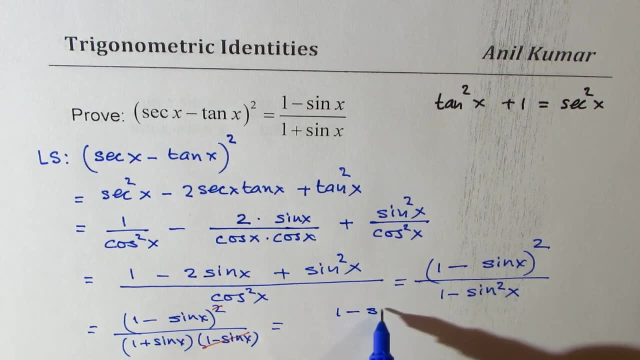 sine x. Correct. Now one of the factors get cancelled: 1 minus sine x. What remains is what we need, which is 1 minus sine x over 1 plus sine x, Correct. So these two factors remain, and that is the right side. 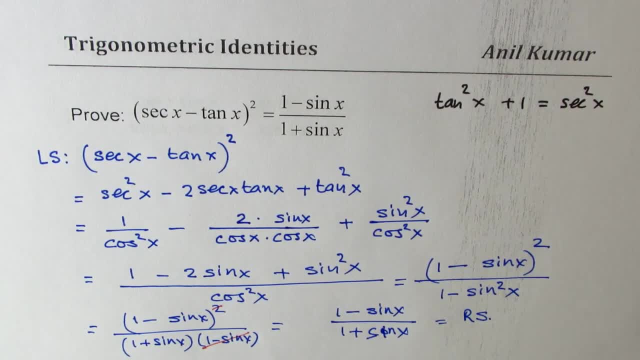 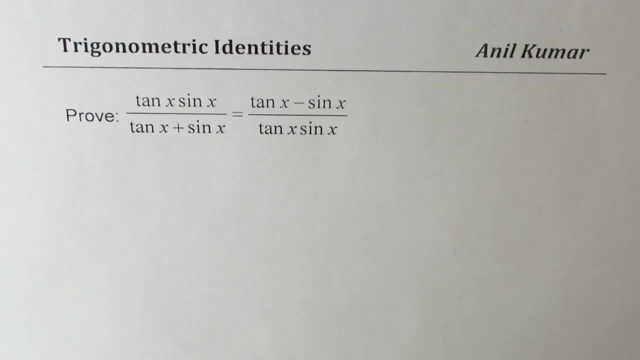 So we have again shown that left side is equal to right side and that is the way to go about, Correct. Now here is the last identity to prove: tan x sine x over tan x plus sine x equals to tan x minus sine x over tan x sine x. 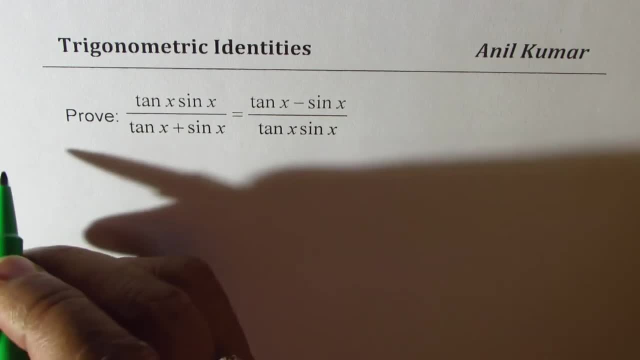 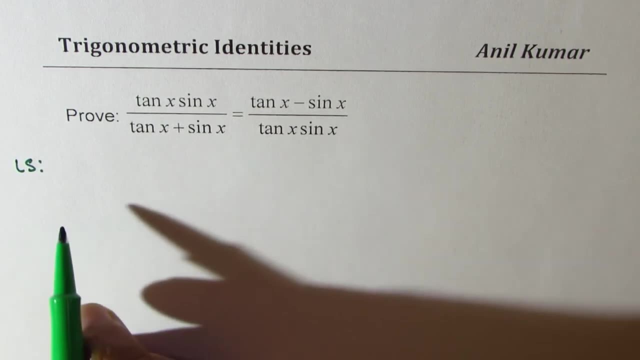 Now let me adopt a different method here. So what I will do here is start with left side and we'll prove that this is equal to something, and then we'll start with the right side and we'll prove that that is also equal. 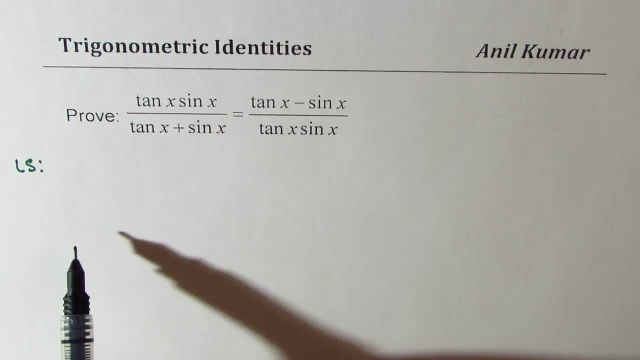 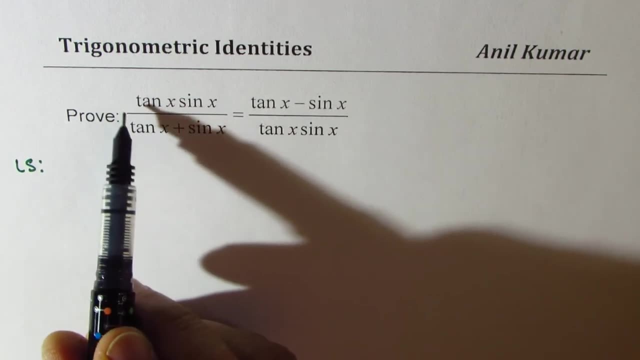 to the same thing. So this is the strategy which we are trying to follow. So first step here is from the left side, which is tan x sine x over tan x plus sine x. I'm going to write them in terms of sine and cosine. 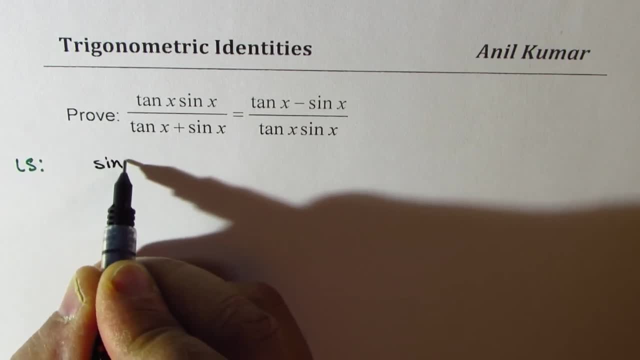 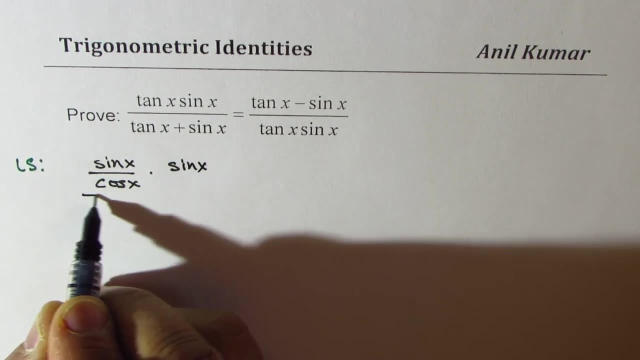 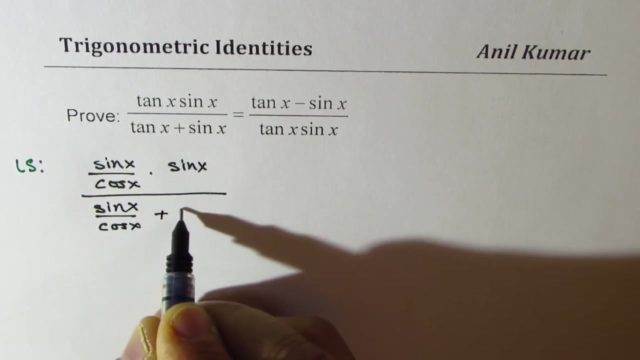 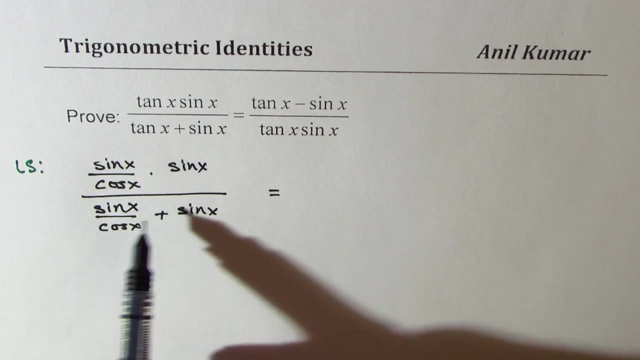 Correct. So tan x can be written as sine x over cosine, Correct. And here we have sine x correct, Divided by tan x plus sine x means sine x over cosine x plus sine x. Now what we can do here is we have sine squared x over cosine x, correct. 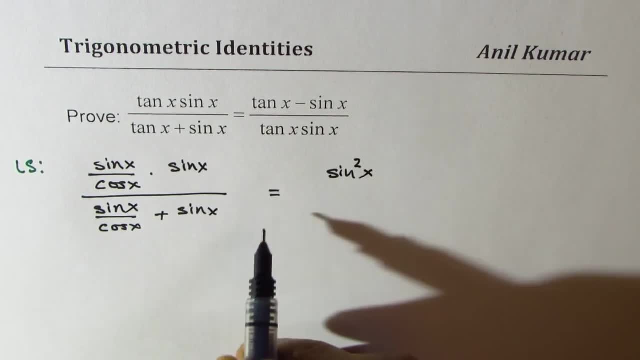 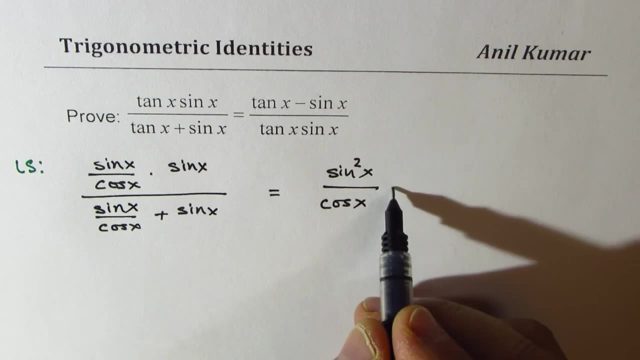 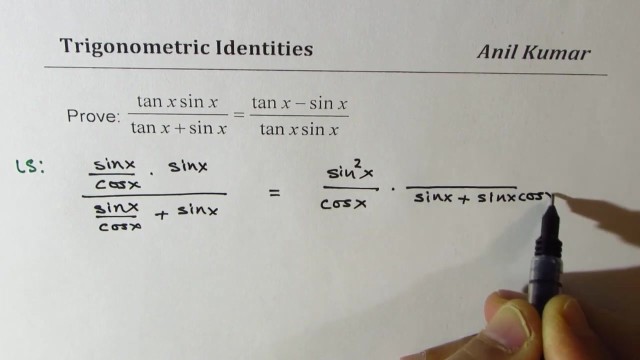 So we have sine squared x here And this cosine x I'm writing in the denominator. Do you see that Cos x In the denominator I have? I will take common denominator cos x. So at present I will write this as sine x plus sine x, cos x divided by cos x. 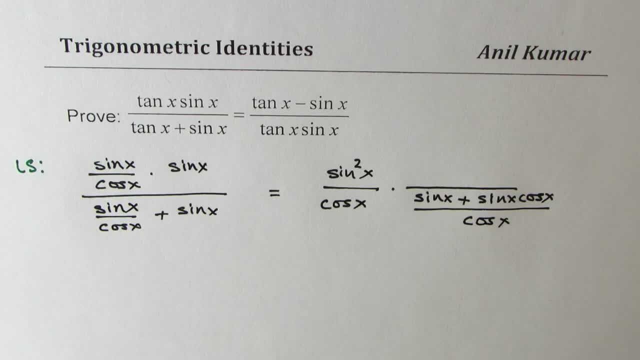 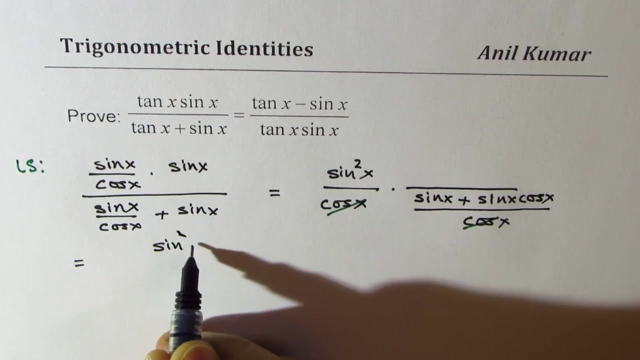 Correct. So I've taken cos x common and then you could cancel these two cos x. You get it Right. So you get sine squared x over sine x plus sine x, cos x. Now I could write this as sine squared x over. I can take sine x common. 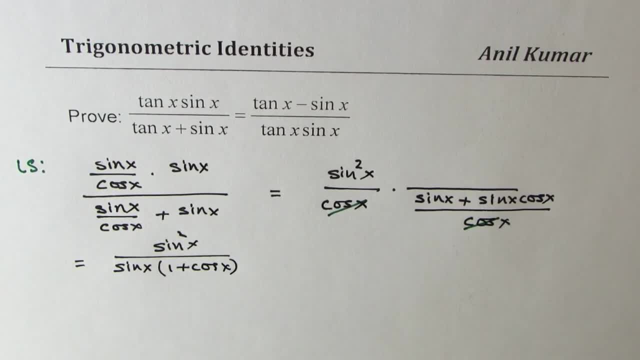 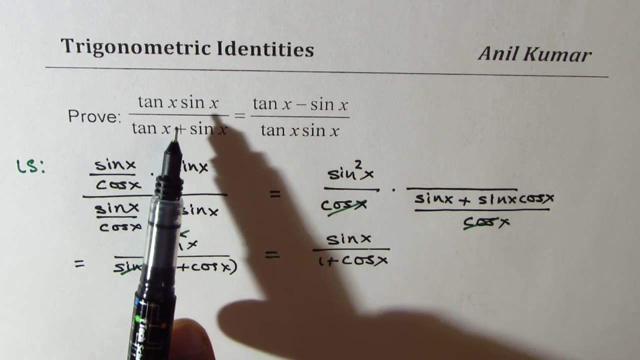 So I get 1 plus cos x. Canceling one of these sine x, it reduces to sine x over 1 plus cos x. Correct, Sometimes we just ask half of the question, That is, this side is equal to that. 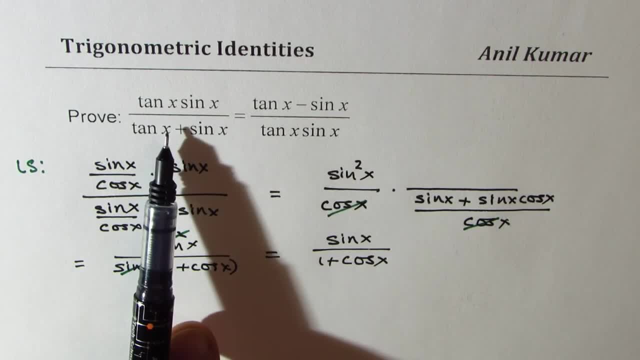 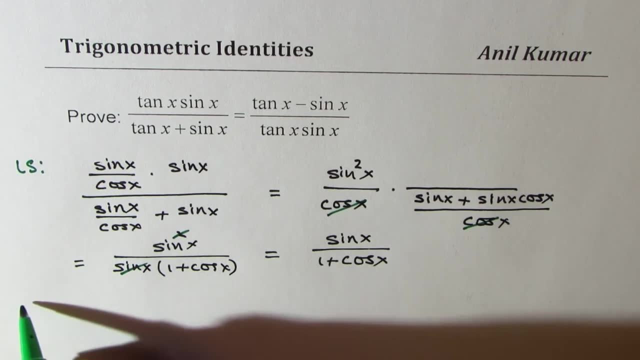 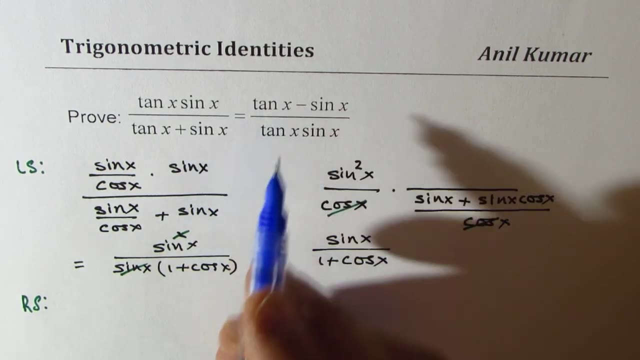 And that's the reason why I'm doing like this. You could actually get a question which is: the left side equals to sine x over 1 plus cos x, Correct, Now let's work on the right side. So right side for us is tan x minus sine x, this time. 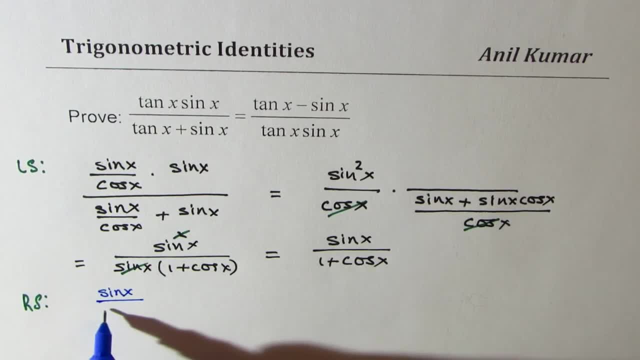 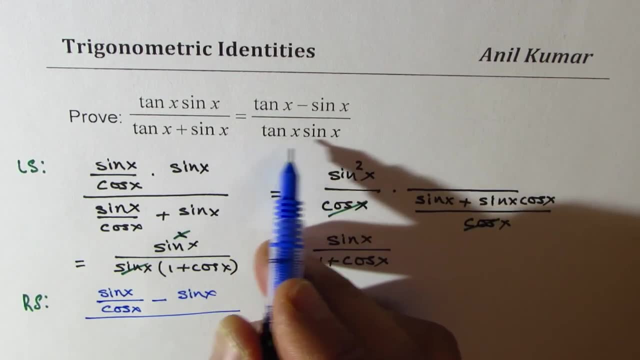 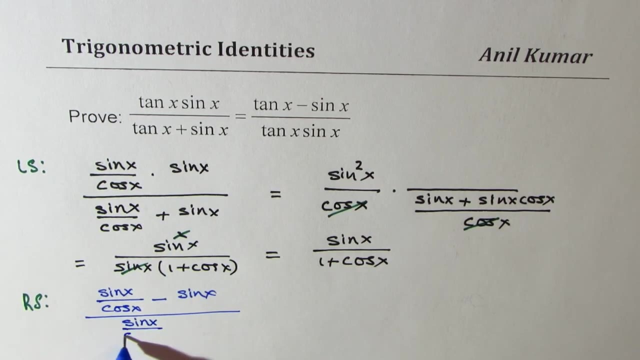 So it could be written as sine x over cos x minus sine x, Correct. And the denominator is their product: tan x sine x, just as we did here. Correct. So the denominator could be written as sine x over cos x times sine x. 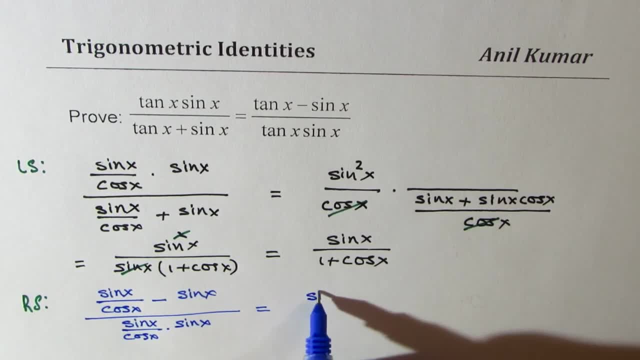 So, as we did here, cos x is the common denominator, We get sine x minus sine x, cos x over. so let me write this as over: cos x, Correct Divided by, we have sine square x over cos x. So these two denominators, cos x, cos x, cancel away. 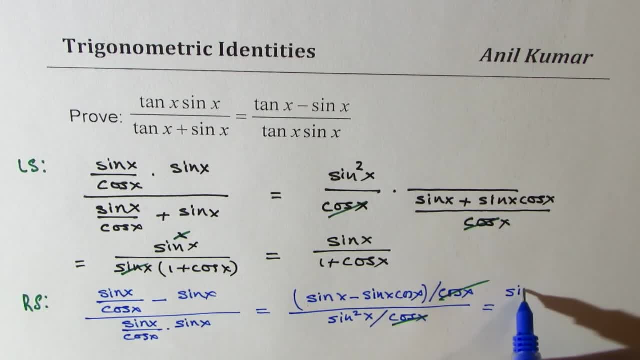 And in the numerator I can take sine x common, giving me 1 minus cos x over sine square x, Correct, So that's the denominator Correct. So when we get this, we could cancel one of these sine x's And what we get here is equal to 1 minus cos x over sine x.